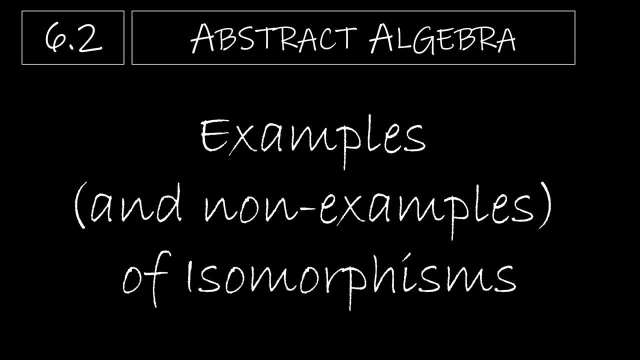 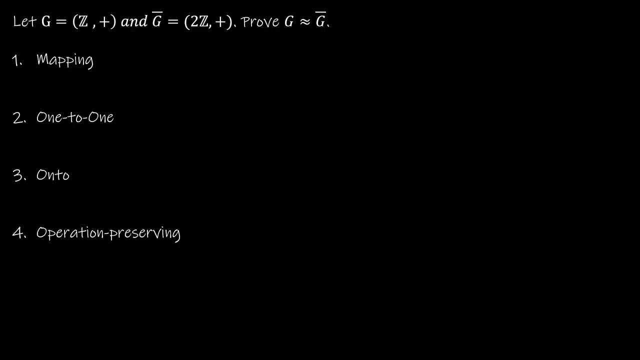 In this second video for chapter six, I just wanted to go through some more examples and some non-examples of isomorphisms. So some group mappings that are in fact isomorphisms and some that are not and why they are not. So make sure that you first watch video 6.1 where we've talked about what an isomorphism is in detail and the conditions that we need to check. And we're going to go ahead and continue checking those details for our first example. This example has two groups g which is the set of integers under addition and g bar which is the set of even integers under addition. So even integers. And we are trying to prove that they are isomorphic. So first thing we need to do is the mapping. Now this is an example of a group of isomorphisms. So we're going to of two infinite sets. So our mapping is not going to list out the values and which value of g maps to which value of g bar. Instead, we're just going to define phi of x to be 2x for all x in g. 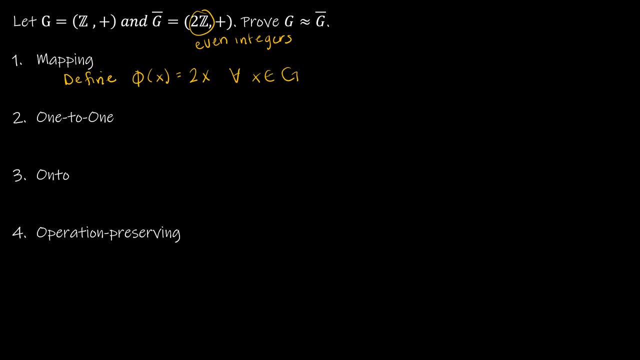 Again, every integer is an integer. So we're going to define phi of x to be 2x for all x in g. We're just going to multiply it by 2 and that will make it an even integer. 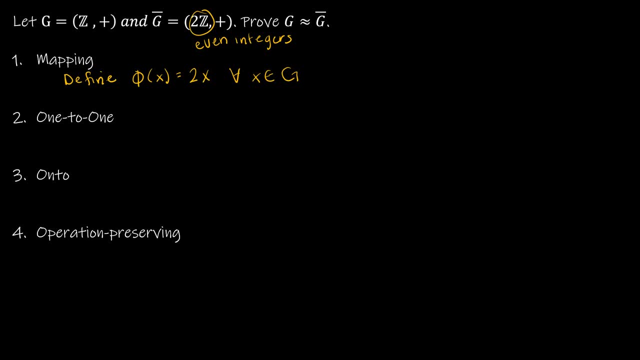 Now, is this one to one? So we're going to let 2x equal 2y. And then by division, we have x equals y. And that is exactly what we were trying to prove. Remember, we assume 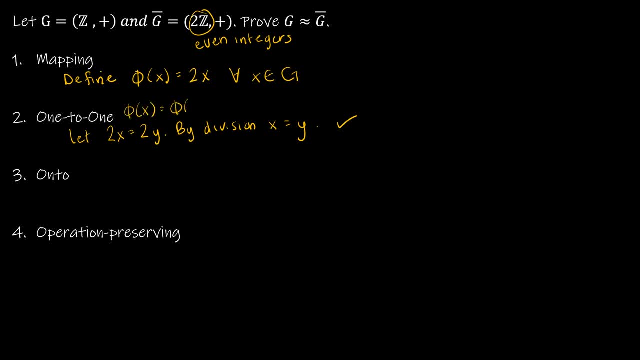 that phi of x, equal to phi of Y and then we show X must equal Y or you can use a and B or L 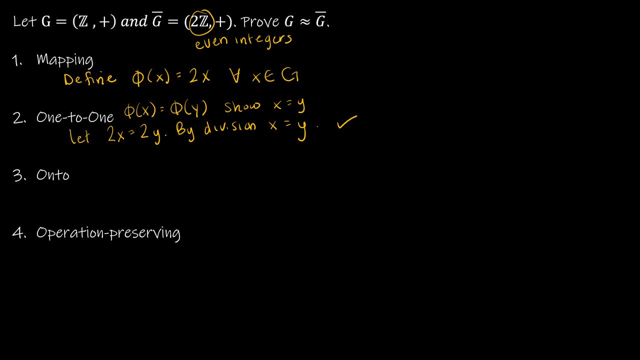 and M it doesn't matter now for onto we are looking for for each Y that is in G bar or each G bar in G bar however you want to say it there must exist an X in G so in our original set our first set such that C of X is equal to Y so essentially what that means is we have to say let Y equal Y so essentially what that means is we have to say let Y equal Y so essentially what that means is we have to say let Y equal 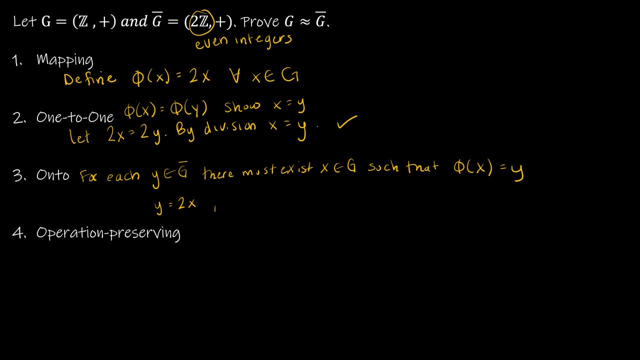 to x, which means x is equal to y over 2. Now that works just fine, but we also have to say, is that going to be an integer? Well, since y is in fact an even integer, remember we're looking at even integers. When I divide it by 2, I will get an integer. So x will be an integer. 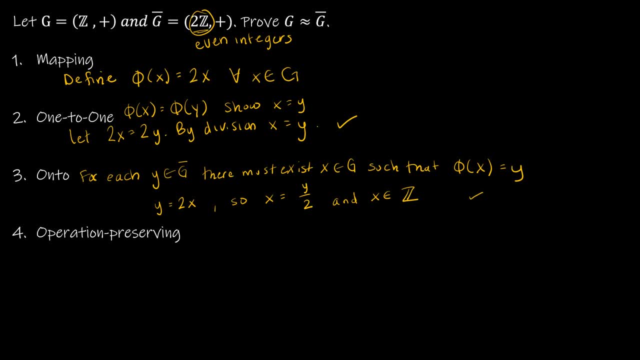 So it is onto. Operation preserving, we need to say that phi, and again, we're dealing with addition, so m plus n is equal to phi of m plus phi of n, or x and y, it doesn't matter what you use. So if I say phi of m plus n is going to be 2 times the quantity of m plus n. Now breaking that down, obviously I can use the distributive property to say this is the same as 2m plus 2n, and 2m is the same as phi of m, and 2n is the same as phi of n. So this is operation preserving. Therefore, g is isomorphic to g bar. Let's look at another example. We have 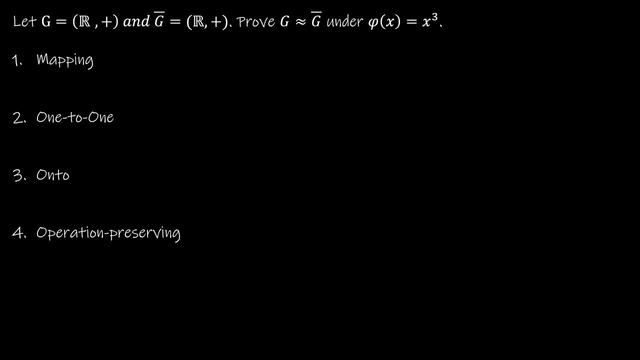 g bar are both a set of real numbers under addition, and we want to prove that they're isomorphic under a specific mapping. So obviously they would be isomorphic under, say, x equal y, or phi of x is equal to y, or phi of x is equal to x. Any of those would work just fine. They're asking specifically for the mapping, and so we're going to say let phi of x equal x cubed. 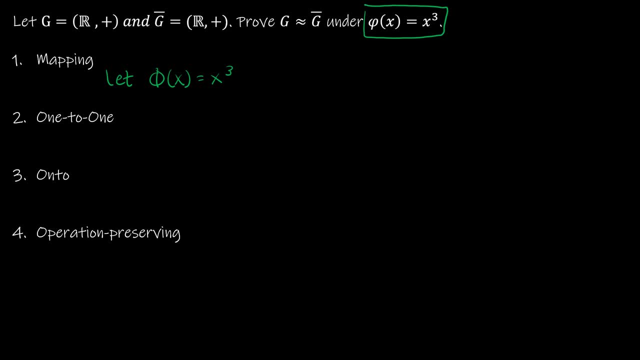 So is this one-to-one? Remember what we tried to do is we are looking at phi of x equal to phi of y, and then we have to show does that imply that x equals y. So back to the discrete math days, it's an implication. So all I'm going to do is say let x cubed equal y cubed, which would be phi of x and phi of y, and then I'm going to take the cubed root of each side, whoops, that's y cubed, and what does that give me? x equals y. So yes, this is one-to-one. 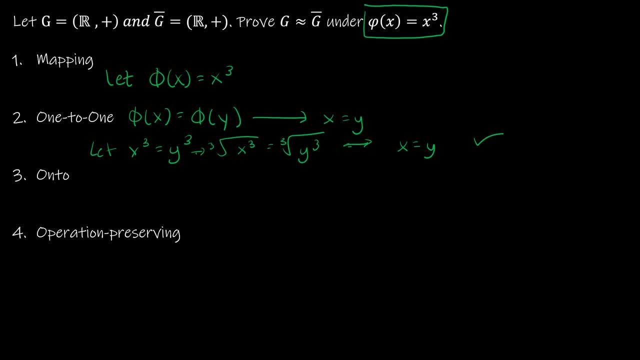 Is it onto? Remember I'm looking for what must, do I have a specific x for each and every y? So I'm really just starting with y equals x cubed, and I'm taking the cubed root of each side, and I'm getting the cubed root of y is equal to x cubed. 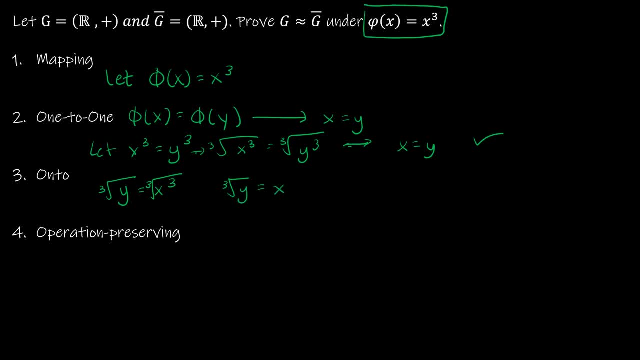 And then remember I need to double check, is x going to be a real number? And just before I continue here, notice I'm not writing out all of the words, so if this were say a homework assignment or if this were a test question, you would use more words. You would say let x cubed equal y cubed. By taking the cubed root of each side, we get x is equal to y. 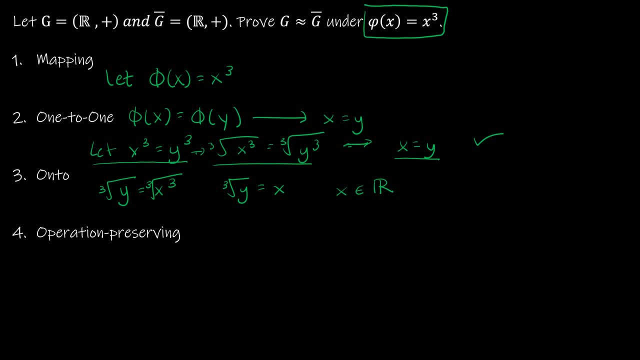 Now I'm going to do the math just to help me. So let's columns X and Y, because $1, or X is equal to Y, and put Y Earth, we get y export from my 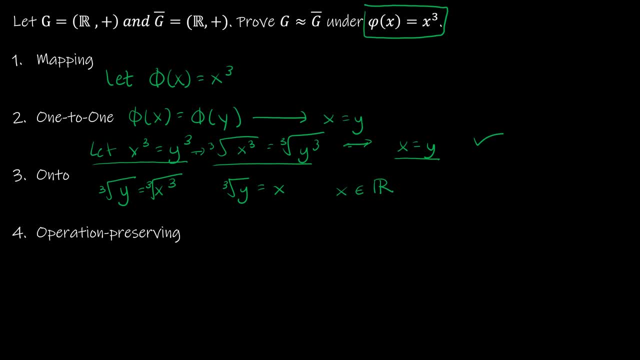 area of 151, 375. So I've got myank 자�, and I've got y новых, whose value is 1 , and I've got other values. I've got the whole problem. OK? 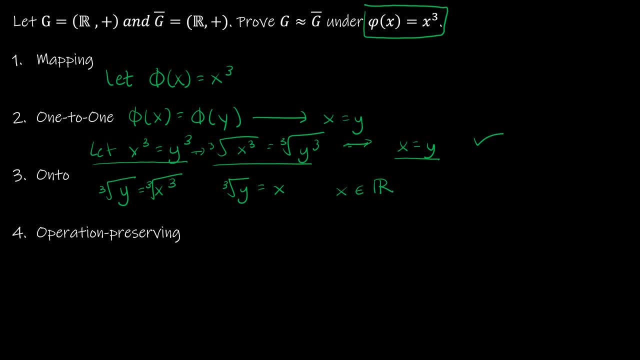 I've got x, square root, then that result is not going to be a real number. It's going to be an imaginary number. But if I take the cubed root of a real number, positive or negative, I am going to get a real, and so therefore this is onto. Now let's take a look at operation preserving. Remember, I'm looking at phi of x plus y, and I need it to equal phi of x plus phi of y. So phi of x plus y means x plus y cubed. I'm saying does that equal phi of x, x cubed, plus phi of y, which is y cubed. Now obviously I could go ahead and multiply this out, but hopefully we know that that is not the case. We can't just distribute this. This side on the left is actually x plus y times x plus y times x plus y, and that is not going to give me x. 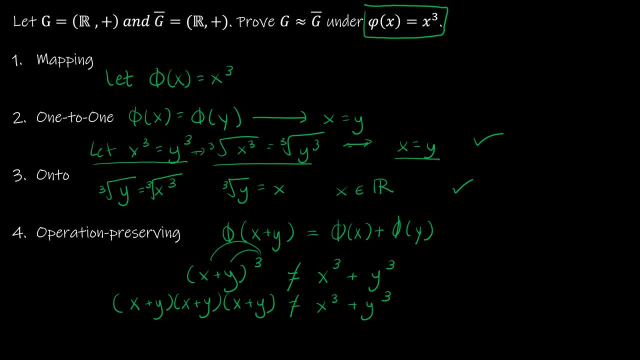 x cubed plus y cubed, because of course I would have to FOIL. I would get x squared plus 2xy plus y squared, and I would take that result times x plus y, and I'm not going to do that. I'm just going to say, no, this is not operation preserving. And again, I knew to use addition because we have addition in our definition of the group. So therefore, g is not isomorphic. 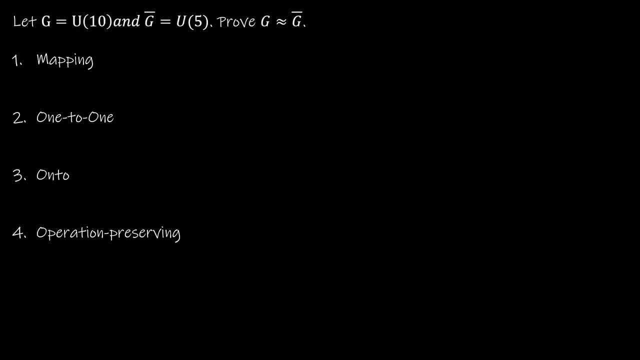 So 2g bar. Let's look at one last example involving u10 and u5. And again, when we're dealing with these u's, we are looking at any value less than n, so less than 10 or less than 5, and relatively prime to n. So if I look at 10, I'm looking at the value of 1, but not 2, since 2 goes into 10, 3, not 4, 5, or 6, 7, not 8, and 9. And if I'm looking at u5, in fact, 1 and 2 and 3 and 4 are all relatively prime to 5. So that's the first good news, because we only have four elements, and because each set has four elements, it's possible that this is going to be an isomorphism. 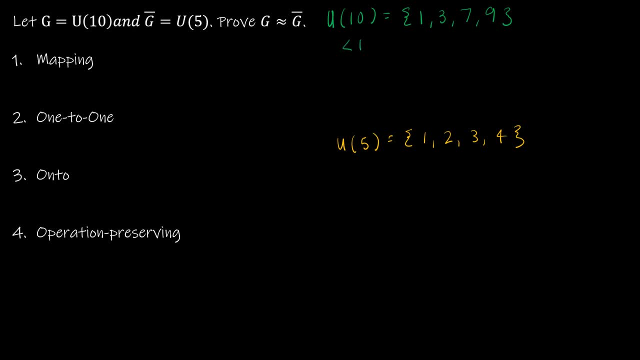 So let's take a look now at each element. So what I need to do is I need to look at each element of the set, and I'm going to look at each element of the set, and I'm going to look at each element 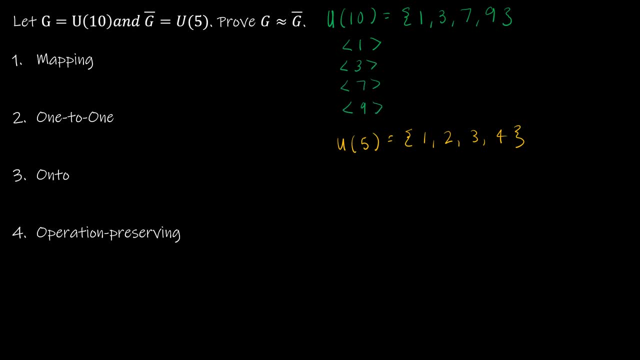 of the set, and in each element, I need to determine the order. So if I am looking at the operation with u, which is essentially mod 10, multiplication mod 10, so I'm looking at 1, and then 1 squared, which is 1, and 1 to the third, which is 1, I only get 1. So the order of 1 is 1. Obviously, that's the identity as well. If I look at 3, I get 3, and then 3 squared, which is 9, and then 3 to the third, which is 27. Again, mod 10 makes it 7, and then 81, which is 1. And that means the order of 3 is 4. And then I do the same with 7. I say 7, 7 squared, which is 49, or 9, 7 to the third, which is 243, and then 2,401, and I end up with the order of 7 being 4 as well. And then for 9, I get 9. 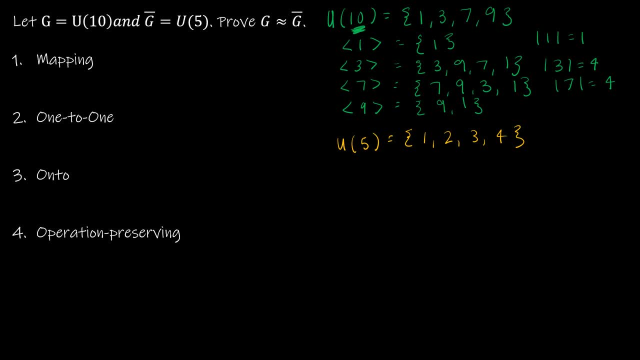 And then 81, and then I believe 729, but it goes back to 9. So the order of 9 is 2. 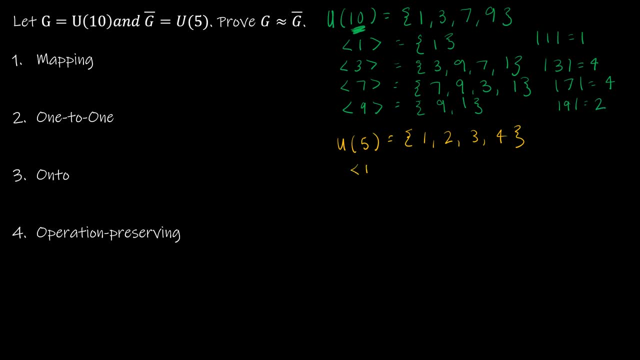 Now let's do the same for the elements of u5. So 1, 2, 3, 4. So 1 still just generates 1, and in fact is still the identity. 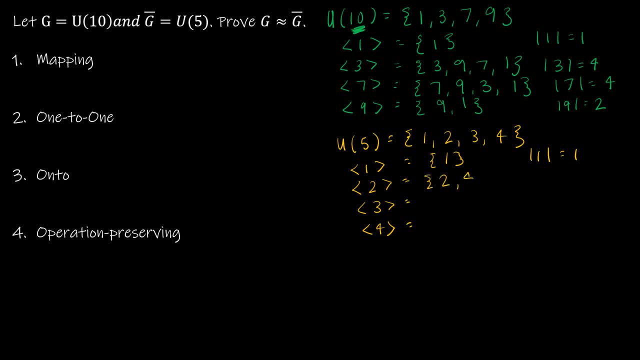 So 1 is 2, 2 squared of 4, 2 to the third, which is 8, but mod 5 this time, 8 would be 3. And then 16, mod 5 would be 1. So that does generate the set. So this is a cyclical set. And that's helpful to know too, because obviously my first set was cyclical with order 4, and this is a cyclical set of order 4. 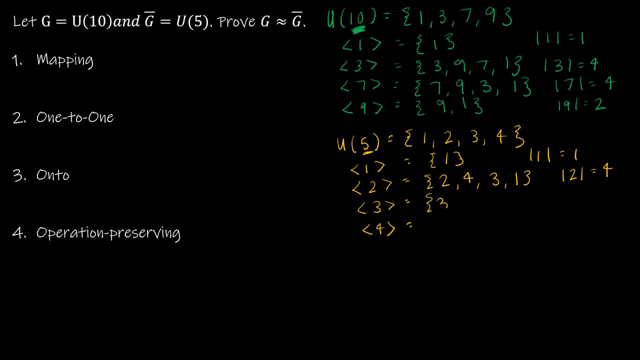 2, sorry, I lost my train of thought there for a second. 3, 3 squared is 9, which is 4. 3 to the third is 27, which is 2. And then 81, which is 1. So the order of 3 is 4. And then I'm looking at 4, which is 4, and then 16, which is 1, and then it goes back to 64, which is 4. So 4 is 2. Now, why is this important? Because when I'm doing my 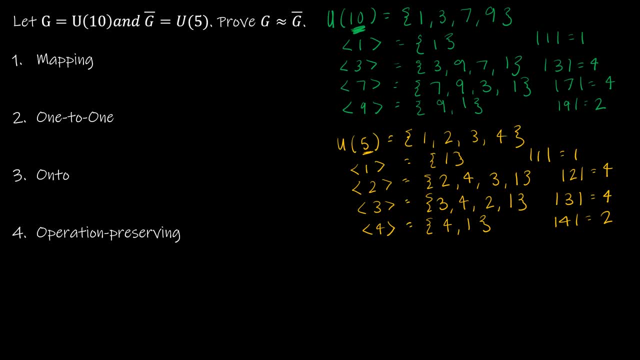 mapping, I have to define which elements map to which. So I'm going to say let phi of, and I have to choose each of these values, so phi of 1, phi of 3, phi of 7, and phi of 9. I have to map each of those to elements of the same order. So 1 obviously has to map 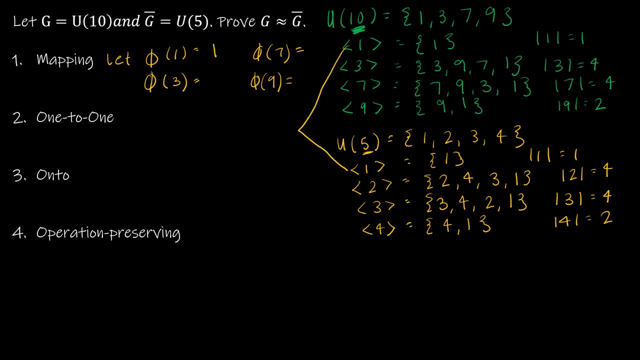 to 1 down here, because they're both of order 1. And 9 has to map to 4, because they're both of order 2. And for the others, it really 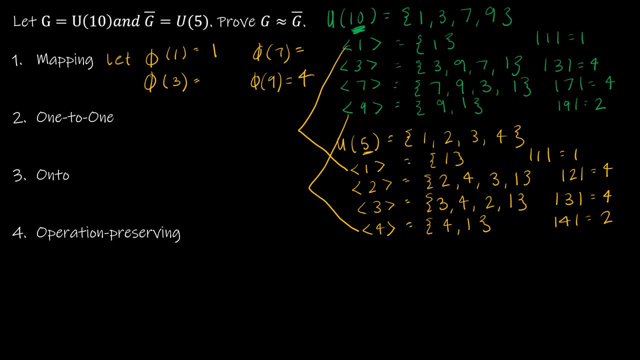 doesn't matter which one you do. So I'm going to go ahead and just say that 3 maps to 2, and 7 maps to 3. Now, 1 to 1 and onto are fairly straightforward, but what I find a lot of students do is that they don't address them at all. So I can say this mapping is 1 to 1. And onto, as shown in the mapping. Because, again, I'm not going to write all that out, but if it's 1 to 1, that means for every x, there's just one y. Well, I've mapped it that way. And if it's onto, for every y, there is an x. Well, again, I've mapped it that 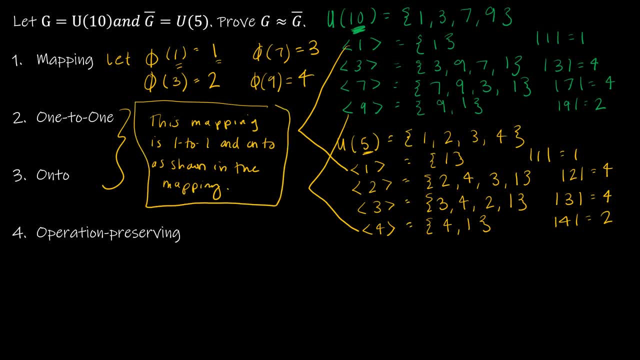 way. So this seems very silly and trivial, and yet if you don't say that you recognize that this is 1 to 1 and onto, then you're not going to be able to do that. So I'm going to say that I'm just going to write onto. 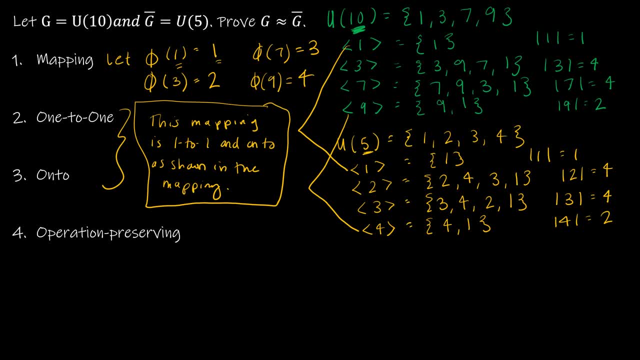 And it looks like I'm going to write onto. So if it's 1 to 1 and onto, then you're going to lose points for it. So just, you know, humor me and give me a sentence that says you realize that you had to check those two properties.